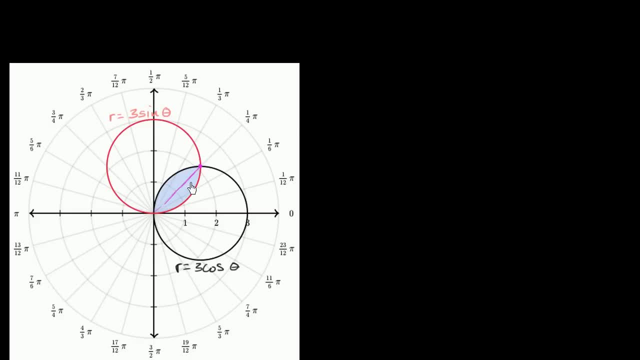 And we can verify that Cosine of pi over four is the same thing as sine of pi over four. So it is indeed the case that these two things are going to be equal to each other. Their point of intersection happens at theta is equal to pi over four. 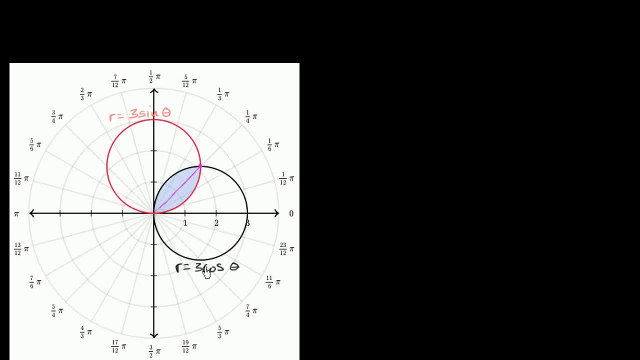 And if that wasn't as important as obvious, you would set these two equal to each other and figure out that theta is where this actually happened. But here it jumps out at you a little bit more. So this is: theta is equal to pi over four. 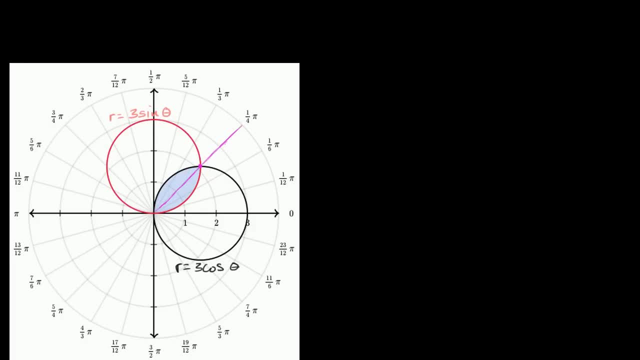 And so the key is to realize is that for theta, theta being between zero and pi over four, we're bounded by the red circle, We're bounded by three. r is equal to three sine theta. And then, as we go from pi over four to pi over two, 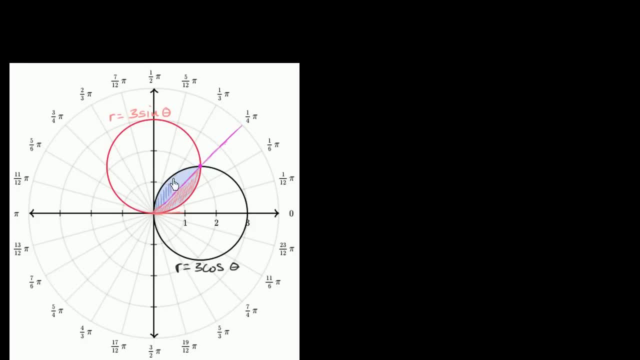 we're bounded by the black circle, We're bounded by r is equal to three cosine theta. So we could just break up our area into those two regions. So this first area right over here we already know is going to be one half times the definite integral from zero to pi over four. 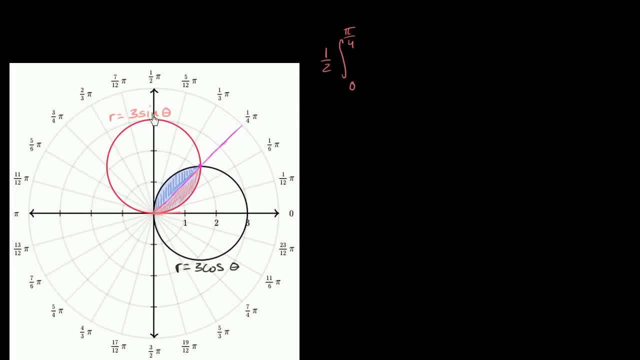 zero to pi over four. of what are we bounded by? Three sine of theta, three sine of theta, And we're gonna square that thing d theta. That's the orange region, And then this, I guess you could say this blue region. 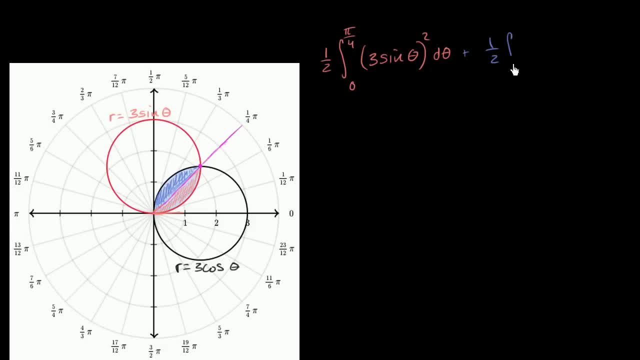 right over here is going to be one half times the definite integral, And now we're gonna go from pi over four to pi over two to pi over two of three cosine theta squared d theta. That's this region right over here. Now one thing that might jump out at you: 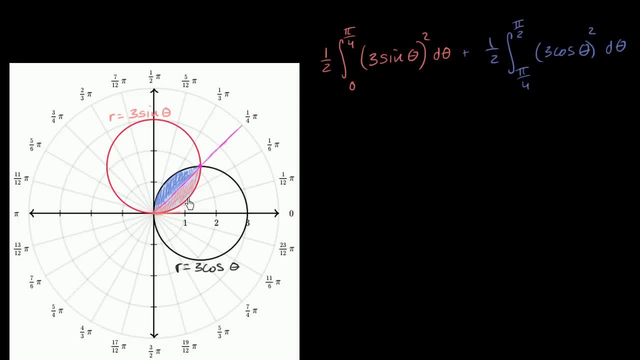 is that they're gonna be the same area, These two circles. they are, I guess you could say, symmetric around this line. Theta is equal to pi over four, So these are going to be the same area. So one thing that we could do is just solve. 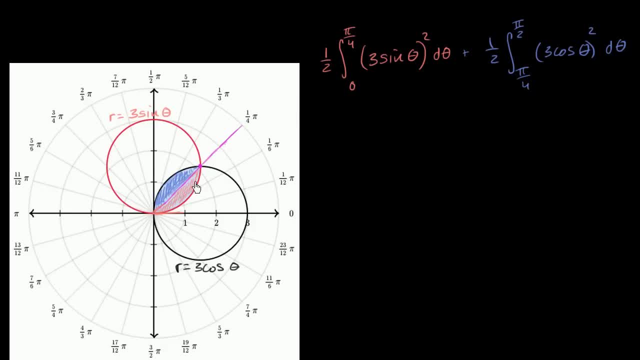 for one of these and then double it and we will get the total region that we care about. So the total area and you can verify that for yourself if you like, but I'm just gonna say that, the total area. I'm just gonna double this right over here. 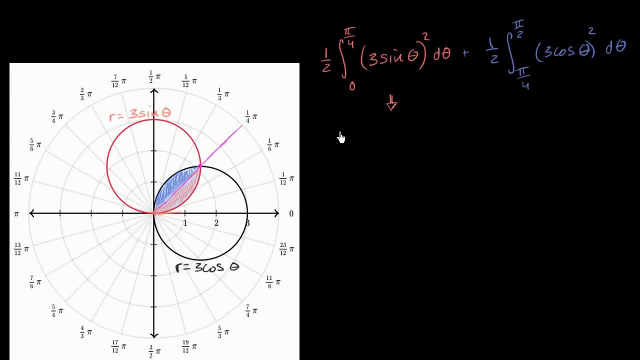 So the total area. if I just double this, just the orange expression, I'm gonna get the definite integral from zero to pi over four of, let's see, let me just of, nine three squared is nine sine squared. theta, d theta. 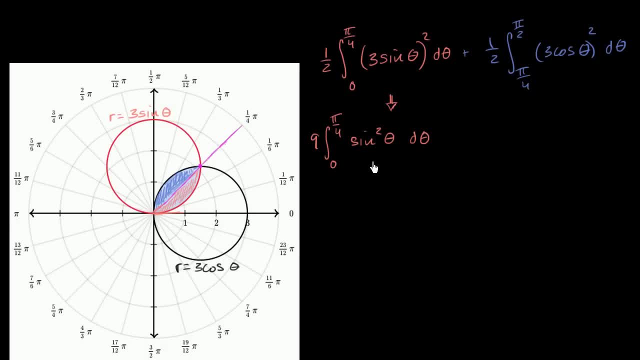 And you could evaluate this by hand. you could evaluate this with a calculator. Let's evaluate this analytically. So sine squared theta is the same thing as one half times one minus one half times one minus cosine of two theta. That's a trigonometric identity. 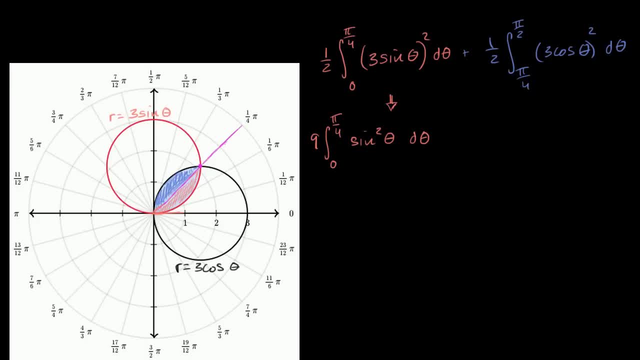 that we've seen a lot in trigonometry class. Actually, let me just write it up here. So sine squared theta is equal to one half times one minus cosine of two theta. So if we replace this with this, it's going to be equal to: 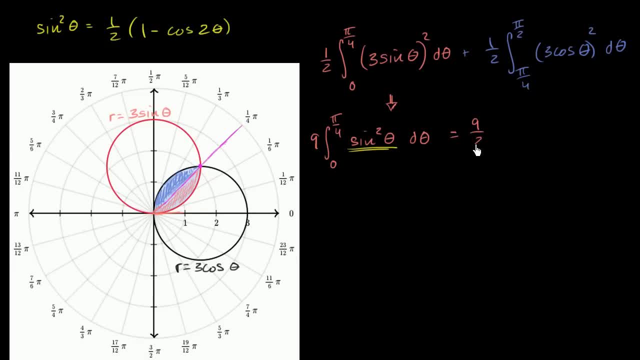 this is going to be equal to. let's take the one half out, So we're gonna get nine halves times the definite integral from zero to pi over four of one minus cosine two, theta d theta, and so this is going to be equal to: 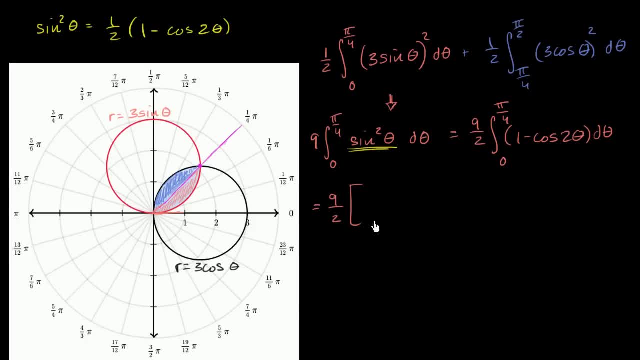 nine halves, nine halves. antiderivative of one is theta and let's see cosine two theta. it's going to be negative sine of two theta. Did I do that Negative? negative sine of two theta over two, over two. 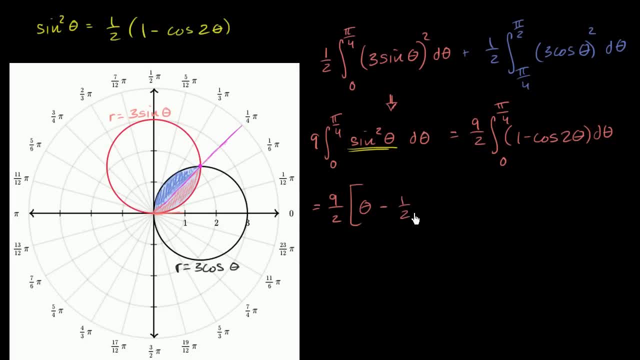 Actually let me. so this is negative one half sine of two theta and you could do u-substitution and do it like this. but this you might be able to do it in your head and you can verify The derivative of sine of two theta. 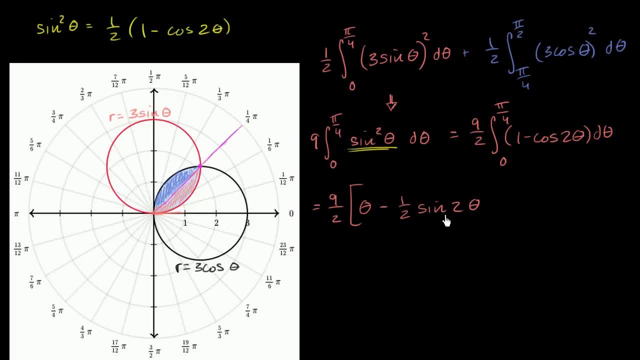 is going to be two cosine of two theta, and then you multiply it times the negative one half, you multiply it times the negative one half. you just get a negative one right over there. And so then we are going to evaluate this at pi over four and at zero. 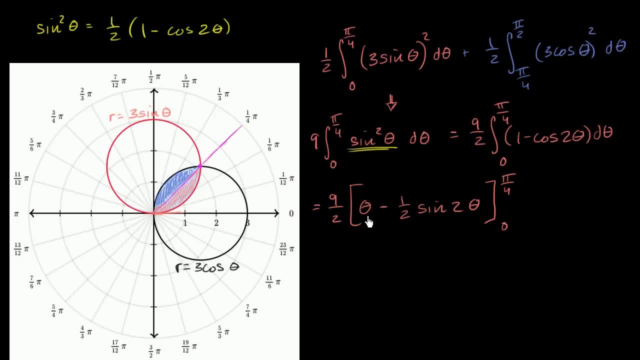 So if you evaluate it at well, luckily, if we, let's see, if we evaluate this thing at zero, this whole thing is going to be zero. so we really just have to evaluate it at pi over four. So this is going to be equal to nine halves.